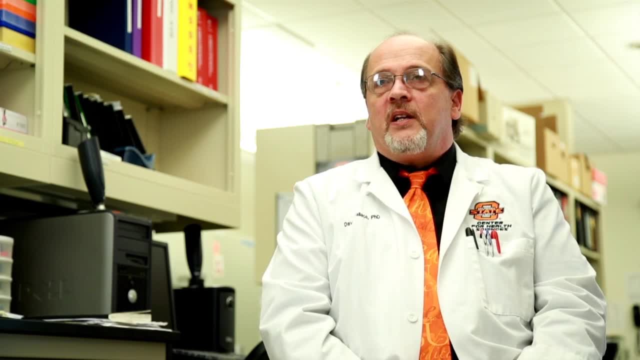 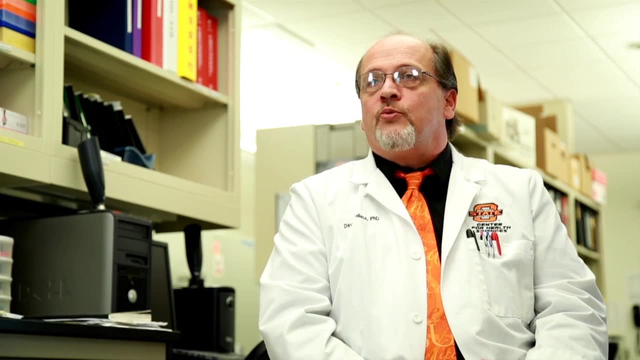 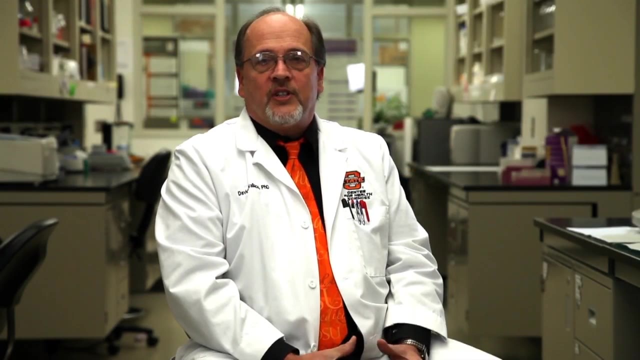 about the effects of cadmium. that was a big news blip a while back, looking at cadmium that was in the paint on children's toys that actually could be leaching out and getting into the child. There's two main focuses within that main project, The first focus being the 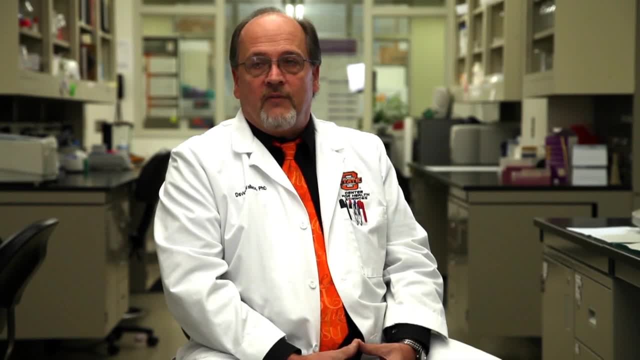 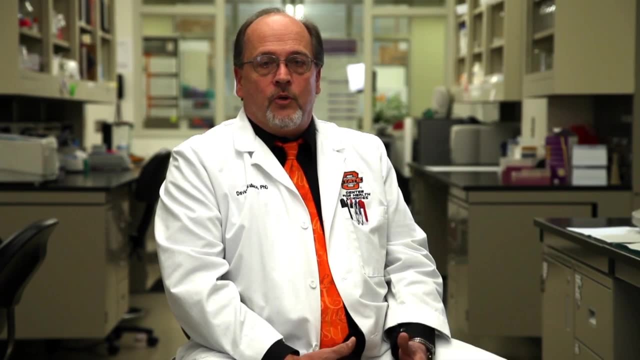 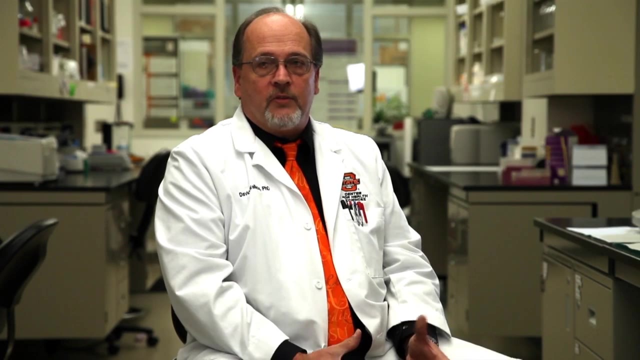 effects of the pesticides and heavy metals on brain development. In particular, we're interested in unborn children who could be exposed in the womb to these pesticides and heavy metals which may or may not accumulate in the unborn child and, in effect, brain development. The second focus is 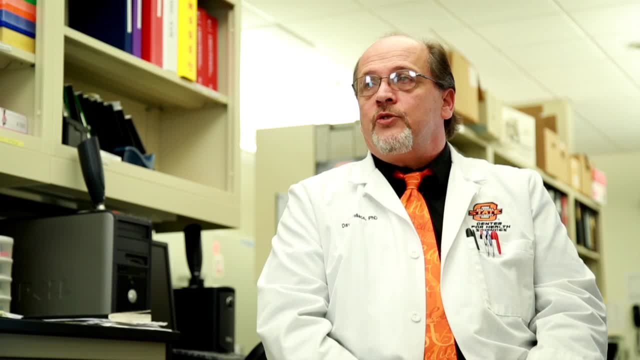 on the effects of the pesticides and heavy metals on tumor development, where most, or a lot, of these chemicals that we're interested in have been reported to be harmful to the brain. The second focus is on 멼'e, these low concentrations of. then we can think about slightly multiple persons whose 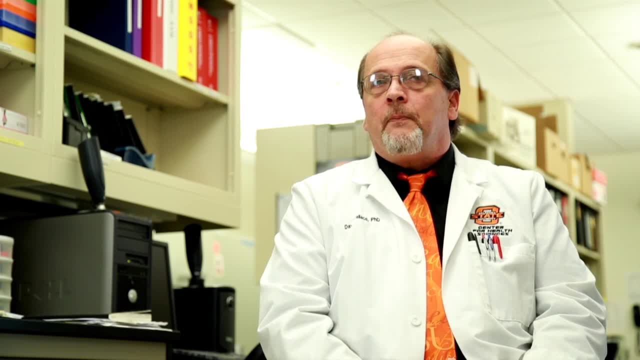 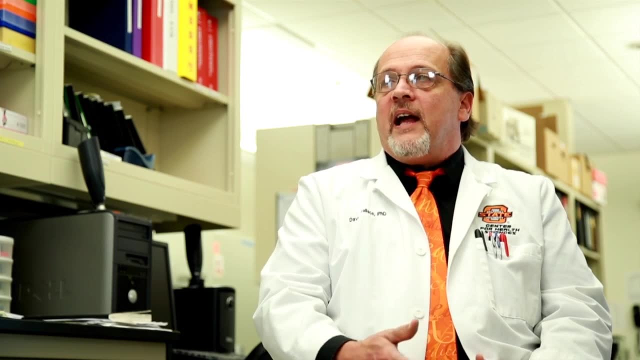 presence, the to a 감eren activity for a long period of time. So what we're trying to do is mimic what you would normally see in the environment and then find out how their staff. there are changes that are occurring. Why we do that is we want to fully understand, or more fully understand the. 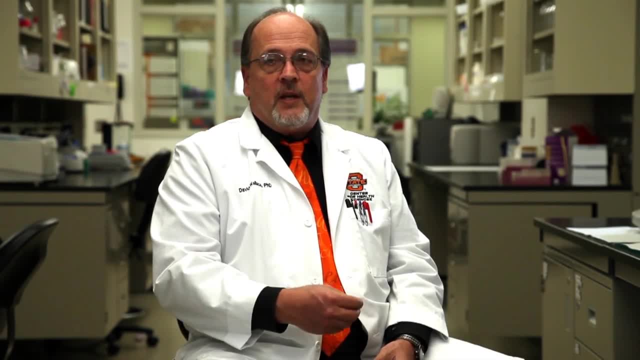 preparation of these disorders? How does the brain alter its development? How does tumor performance impact these disorders? We're interested in wondering how will cancer-based diseases affect brain development? And then why should we try to inspire or encourage changes in the umbrage development and 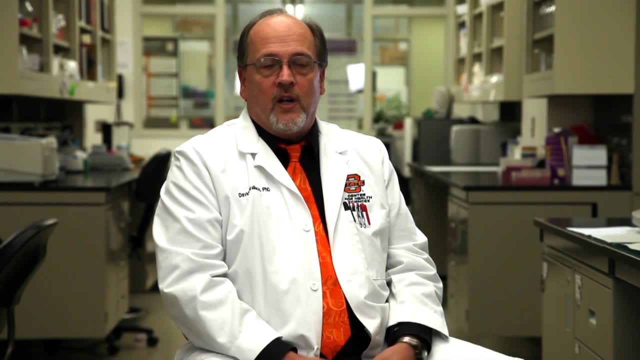 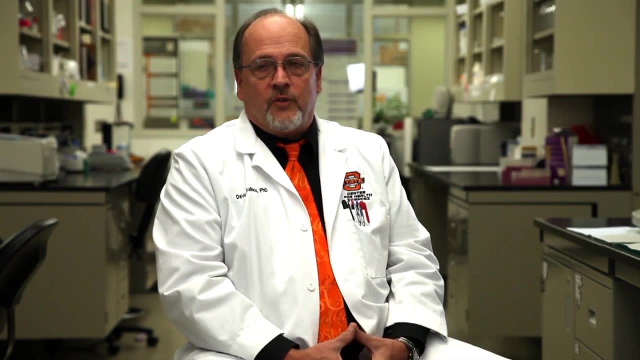 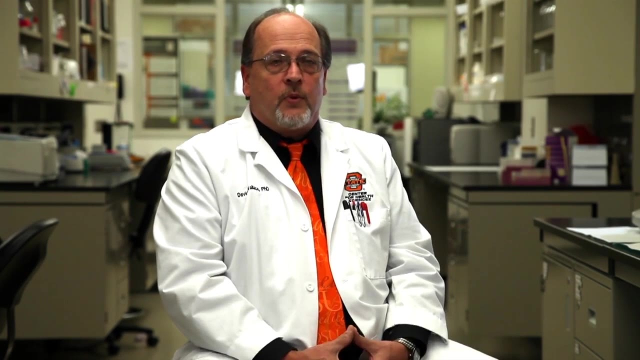 development of estos development occur and if, during this time of exposure, we can figure out certain key points, we can have pharmacological interventions at those points and either prevent the alterations or changes in brain development, as well as prevent the growth of tumors and, ultimately, our goal. 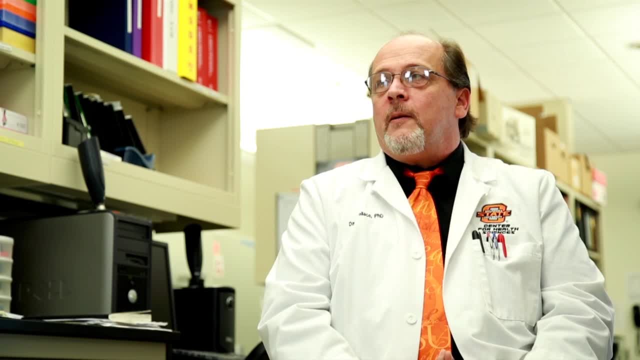 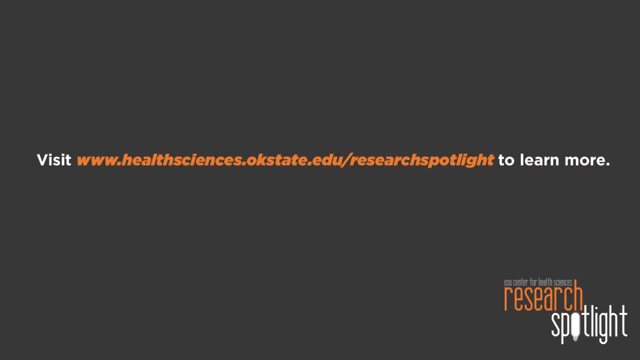 is to improve the quality of life and to improve the pharmacological or medicinal interventions to prevent the development of these disorders.